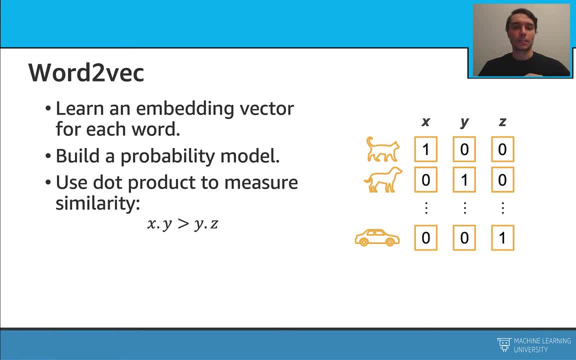 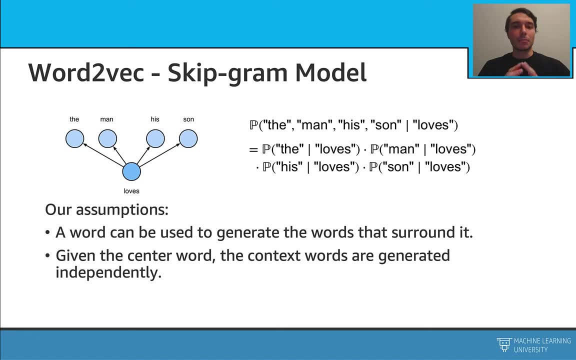 car, we will see a large number. Let's start with the skip-gram model. The skip-gram model assumes that we can create some surrounding words using a center word. With this assumption, as this is a probabilistic model, we will try to write down some probabilities and also try to calculate them. For example: 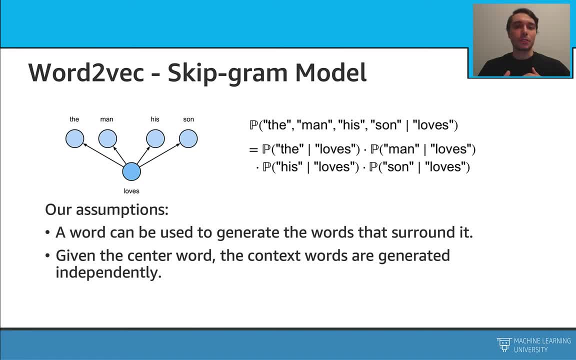 for the sentence demand loves his son. we will try to calculate this probability that for a given word, center word loves- What is the probability that we will see these context words demand his son? So we also have another assumption here. The other assumption is that given the center, 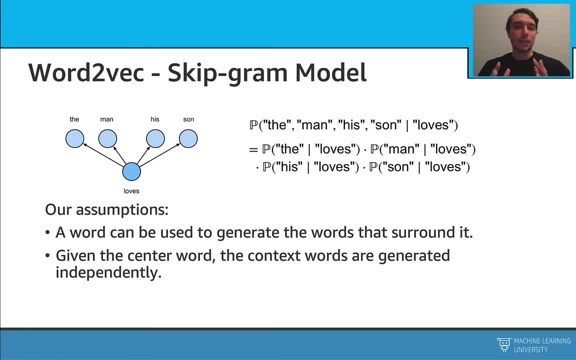 word. we can actually calculate these surrounding words independently By using the second assumption. this actually allows us to break down this probability calculation into smaller pieces so that we can easily calculate. In this case we are going to get these probabilities, the probability that the center, given that the center word- loves. what is the probability? 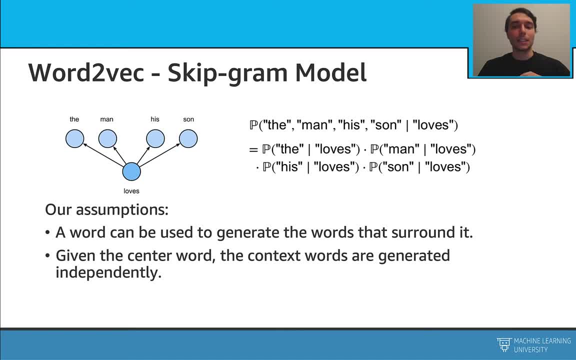 of seeing the around it, For example, times the same situation where we have the center word loves what is the probability of seeing demand, And it goes on like that. So we can calculate this probability in an easier way And this is going to be useful further. 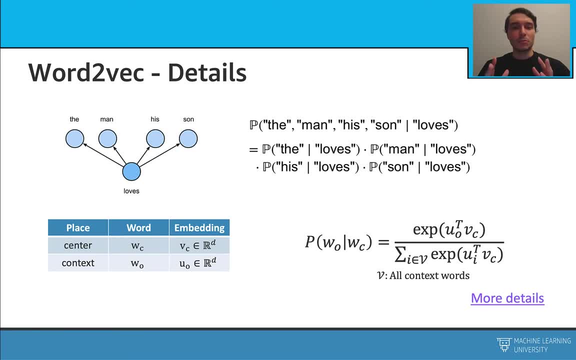 Let's see more details. The full implementation details will not be covered in this class as it is out of scope. Let's see more details. The full implementation details will not be covered in this class as it is out of scope For that. we will only have the details For the. 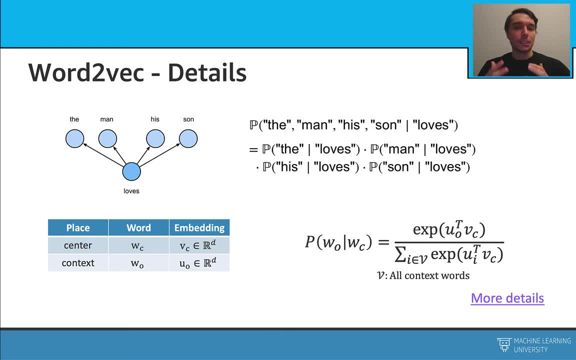 For that reason, I'm going to leave some links for whoever is interested in learning more. So let's continue. We said that with these assumptions we are able to actually calculate these smaller probabilistic terms. Before we get to that, let's also define our word vectors. 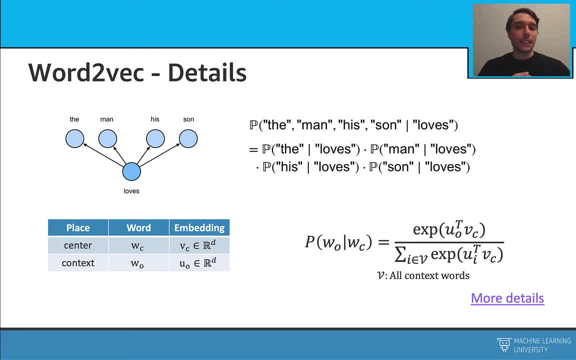 In this setting we are going to have the center and the context as the place where we calculate these things. So we are going to call the center word as wc and the context word with wo, And also we will have separate embeddings For the center word. we will have vc. 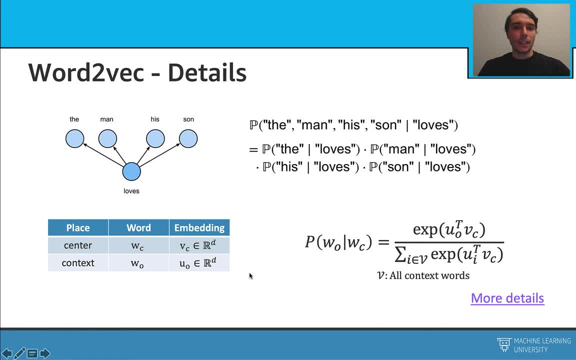 For the context word. we will have uo As a word in a vocabulary can be both in the center and in the context. we will actually have two vectors for every single word. Let's also see how we can calculate this. Just like we mentioned before, we can use dot product to see the similarity between. 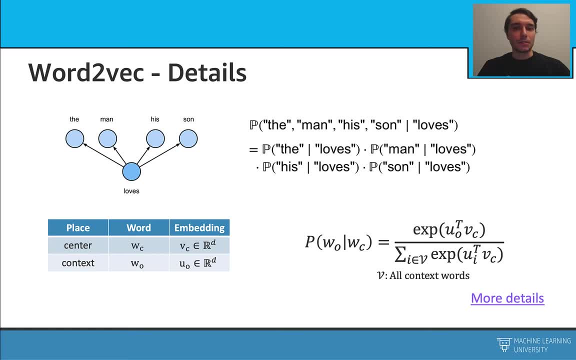 vectors. We can apply the same idea here. For example, we can take a look at the word vectors. We can take the dot product between the center and the context And if this is a large number, it means that they are similar. 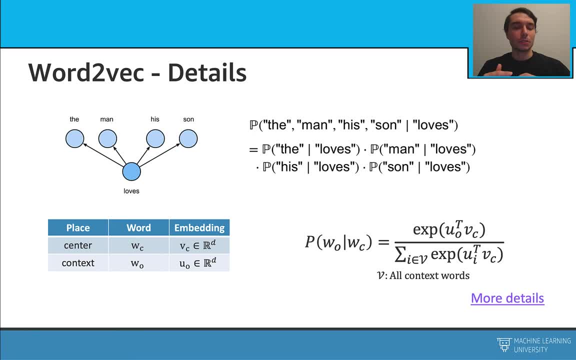 If this is a small number it means that they are not similar. So we can use dot product to measure the similarity. So in this probability calculation Let's see what we can do. We are going to use that idea, But that number is not necessarily a probability number. 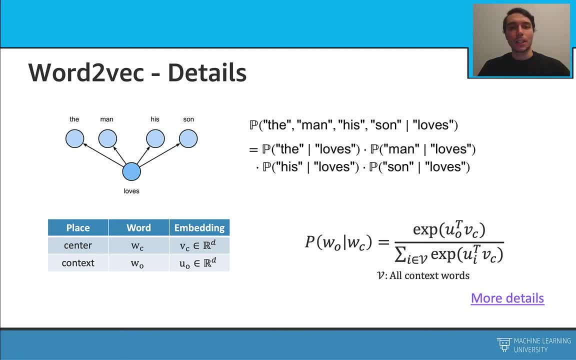 So it's going to be an arbitrary number afterwards. So in order to scale those numbers, we are actually going to use the softmax function here, And in the denominator we will also have this term, where we will also calculate the dot products in this given window. 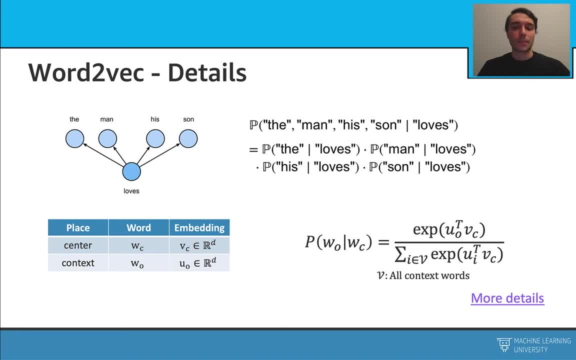 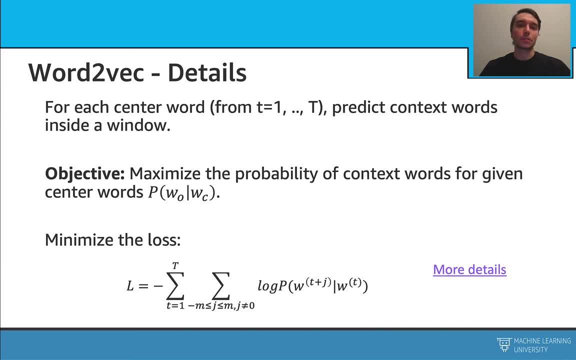 And by using this we are going to be normalizing the term. So in Word2Vec we are trying to correctly predict all these context words for all the center words. So if you try to put this into an objective, we are trying to maximize the probability. 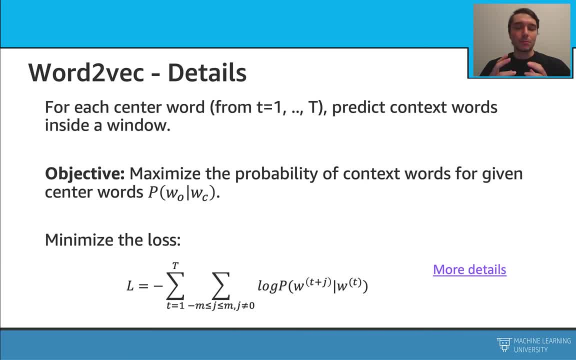 of doing that. There are many more details to the implementation of this, so you can check out the link for that, But we can write this down as a likelihood and from that we can get a loss function And we can try to train a machine learning model with a corpus and try to minimize the. 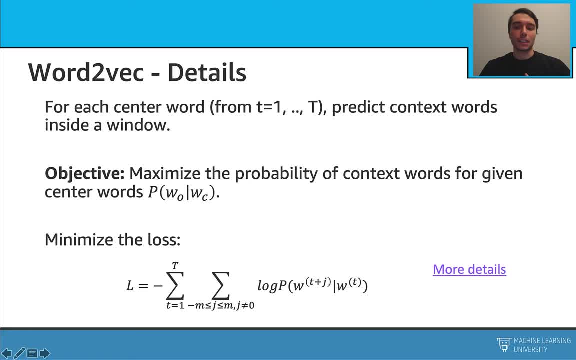 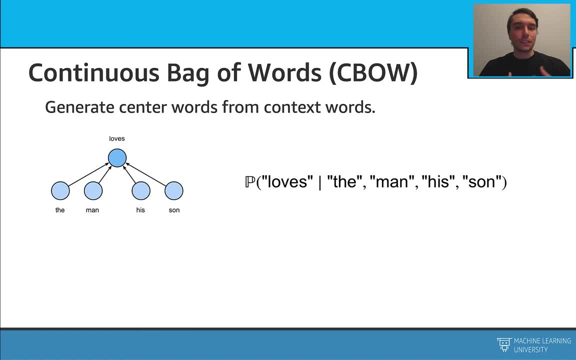 loss function. As I said before, all details are provided in this link. There is also another way of calculating these word vectors, which is called continuous bag of words. In this one, we do the reverse thing. This time we use the context words to predict the center word.